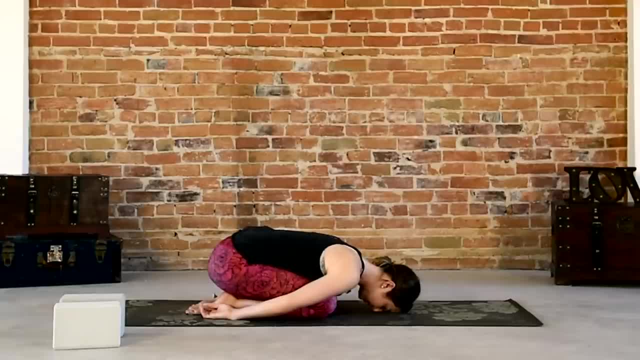 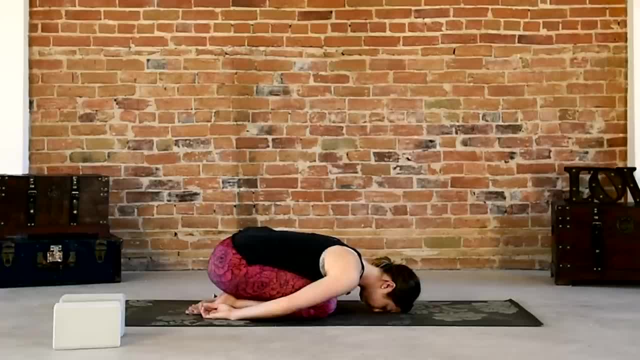 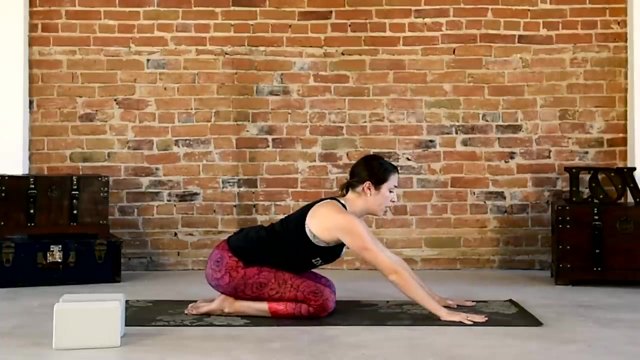 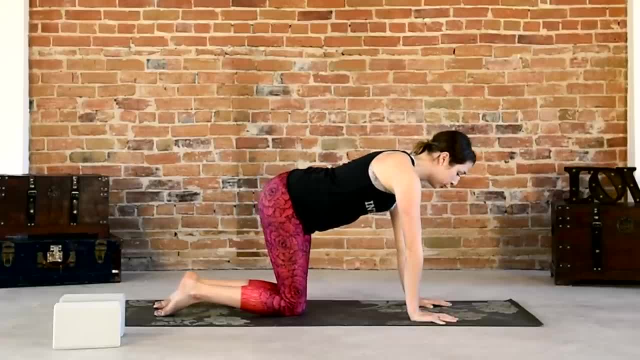 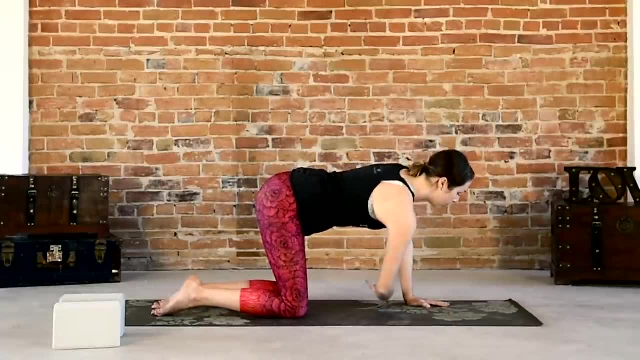 So this is one of the two poses that I found to be the most beneficial for my knot in my upper back. Starting with the right side, you're going to reach your right arm underneath you until the shoulder and the ear either lower to the floor or lower to a block. 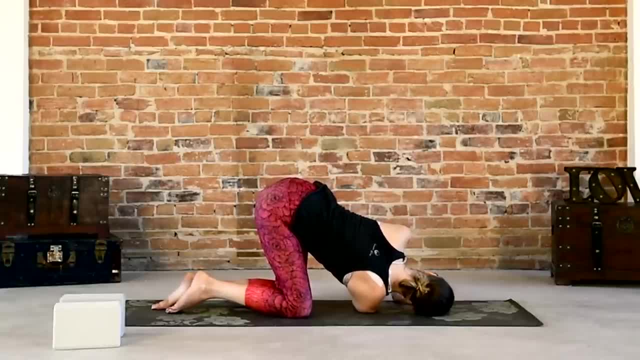 So if the ear doesn't quite make it all the way down, just rest on a block. You really don't want to have to work your neck. Left hand can either stay pressing down into the floor or I find it a lot easier to hold. 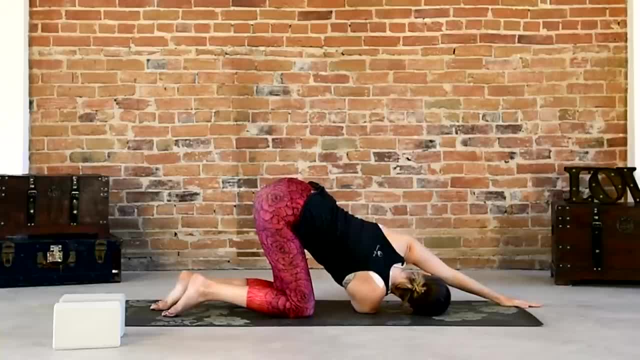 the pose. if I slide my left arm forward, The further you reach your right fingertip, The more you'll feel this in between the shoulder blades and through the upper back. Keep drawing the left shoulder down and away from the ear. This is a bit more subtle, but sometimes when we're in this pose you might notice your. 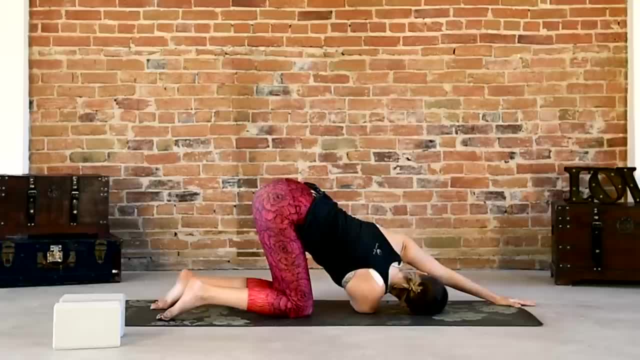 hips are swinging to the left a little bit. Try to bring them back So you're still keeping your hips right on top of your knees. Let the head be heavy, Breathe into the rib cage, Feeling it. Feel it expand front to back and side to side. 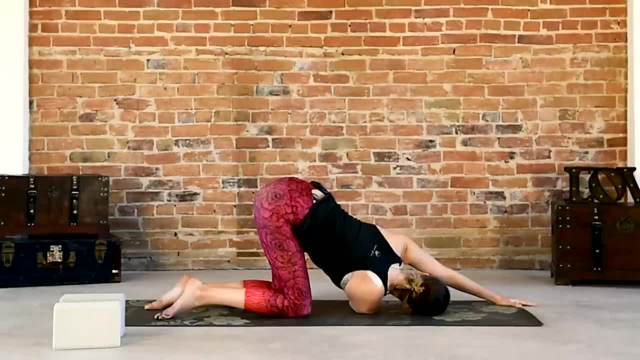 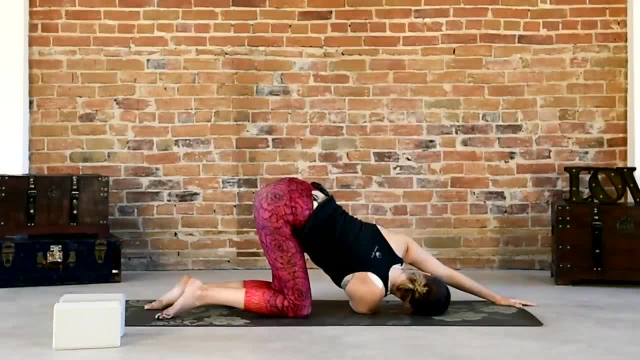 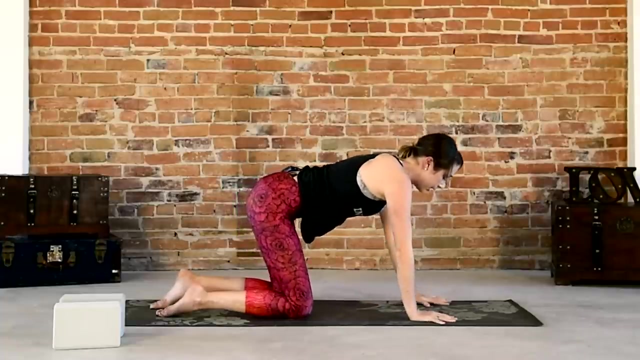 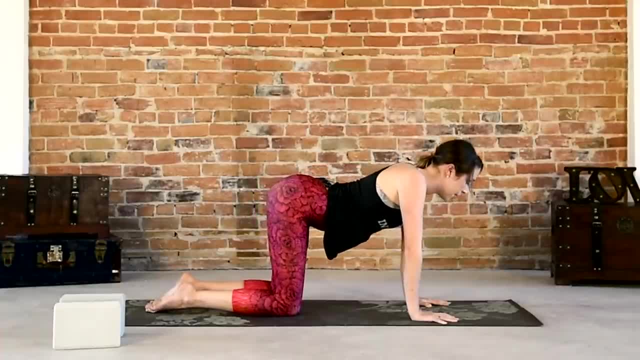 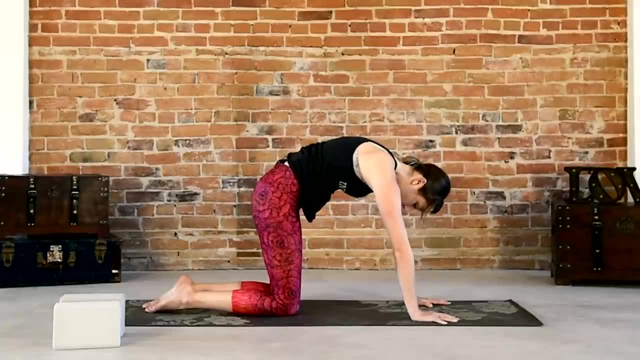 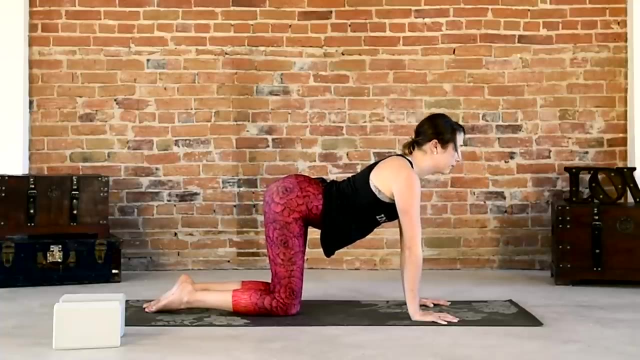 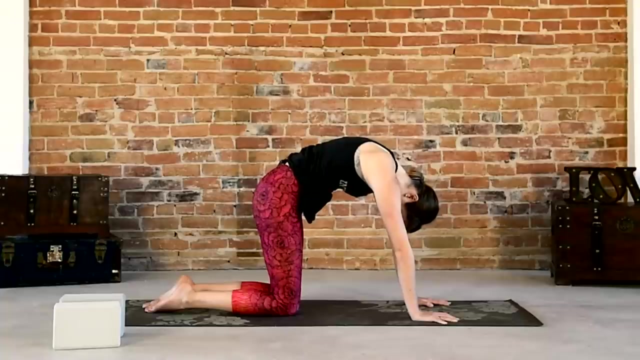 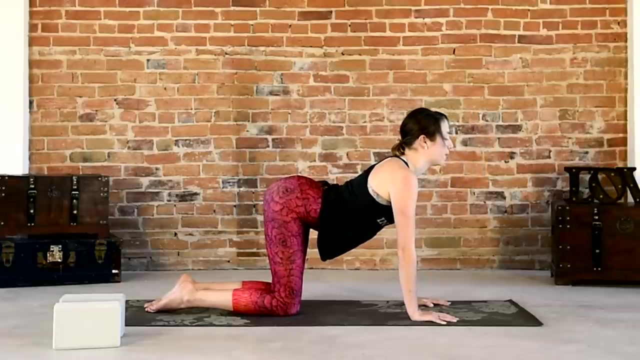 not really exaggerating this movement, making it really gentle. So, inhale, dropping the belly, lifting the gaze. Exhale, rounding the spine, chin to chest. Take a few more. Last one here: Deep breath in And deep breath out as you contract. 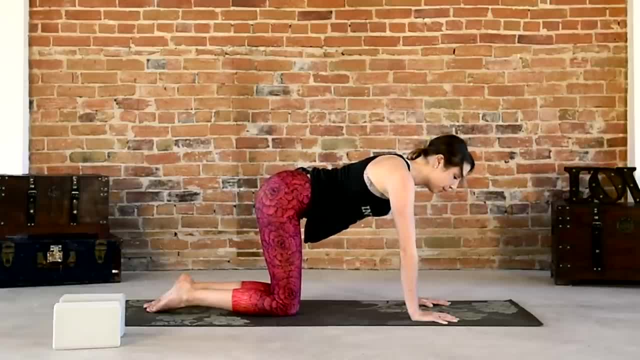 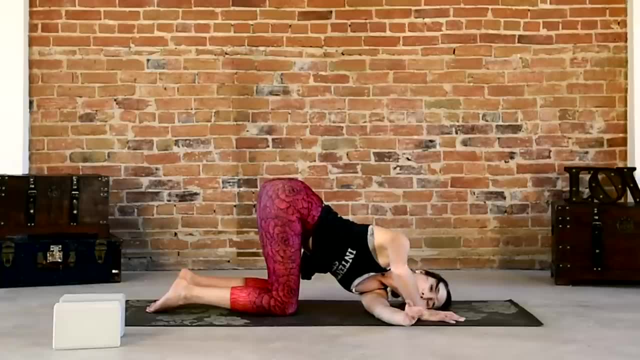 Coming back to your tabletop pose, we'll go to thread the needle on the other side, So this time, left arm underneath you, lowering the shoulder and the ear either right to the floor or onto a block. Relax your neck and either keep your right hand as it is. 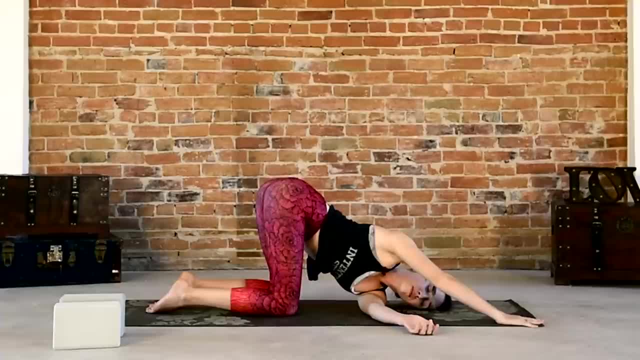 or you can just slide your right hand forward, keeping the elbow relatively straight, drawing the right shoulder down and away from the ear. You might find this a little bit more sensational on one side more than the other, depending on which side you're not. 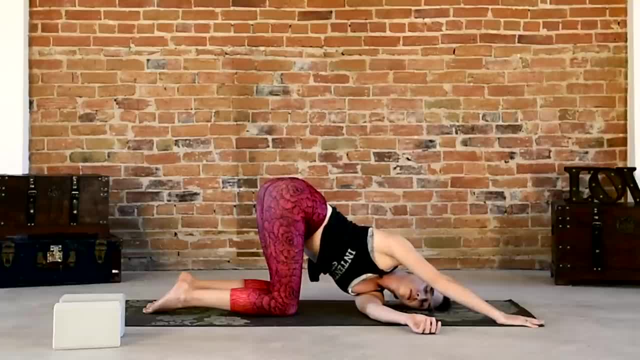 And also this is a very specific pose. It's on the bottom right, Right hand is. You can use your left hip if you want. The other side of the hip is So feel free to back out of the pose at any time that you need to. 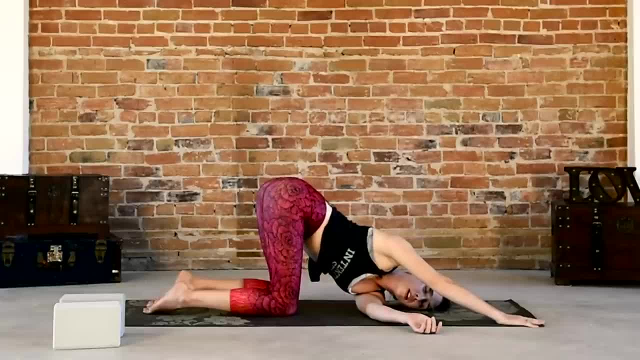 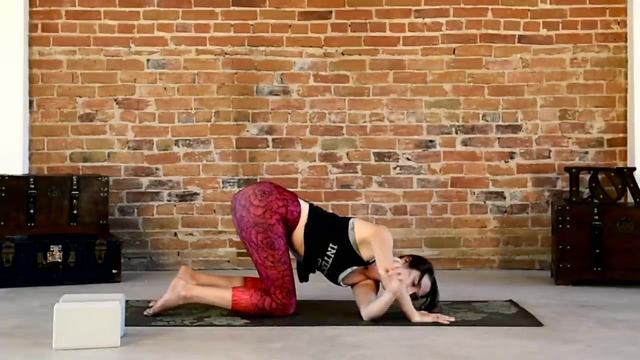 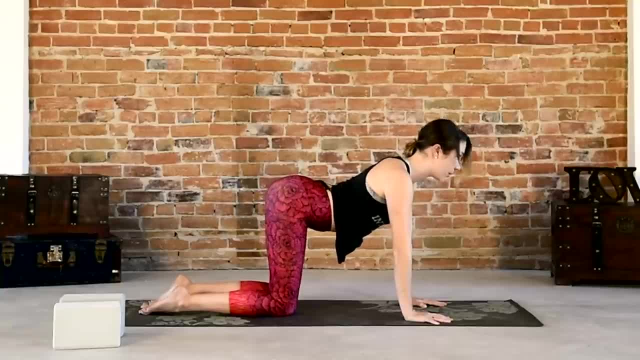 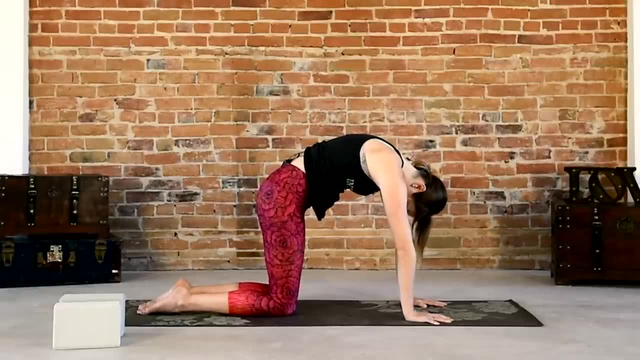 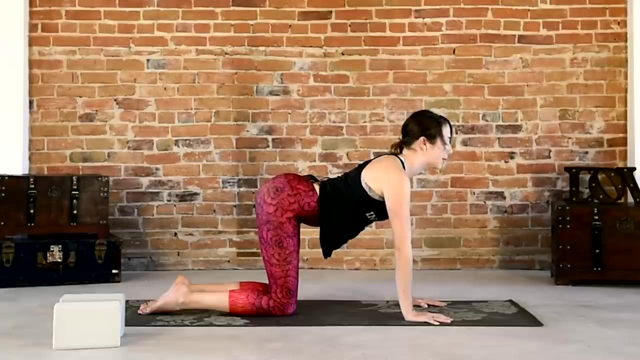 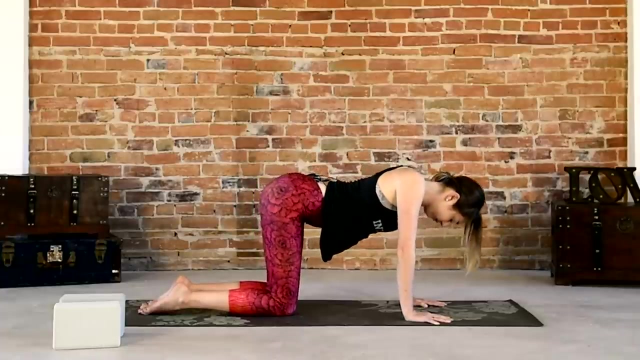 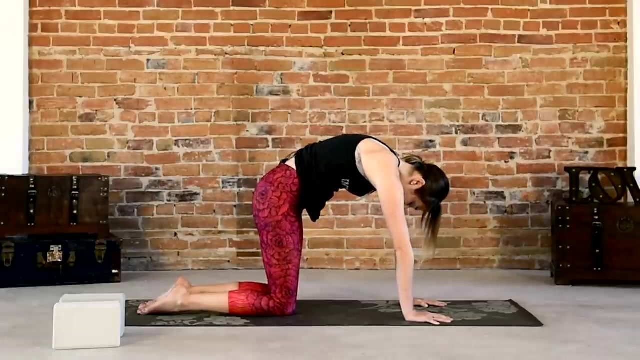 And same thing here: Cat and cowl Inhale, drop the belly, lift the gaze, Exhale round the spine, chin to chest, Moving in and out of those two. Take about two more cycles here And we're going to sit our hips to the floor with our legs stretching out forward, setting up for a straight-legged forward fold. 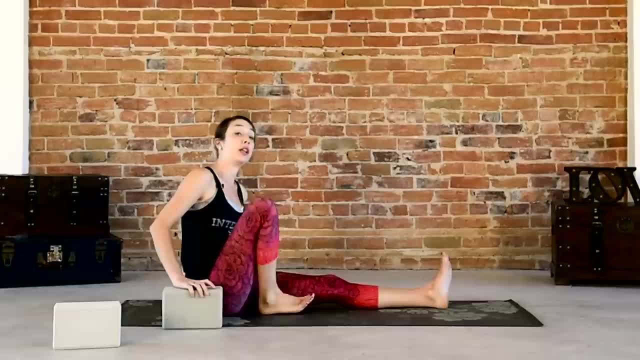 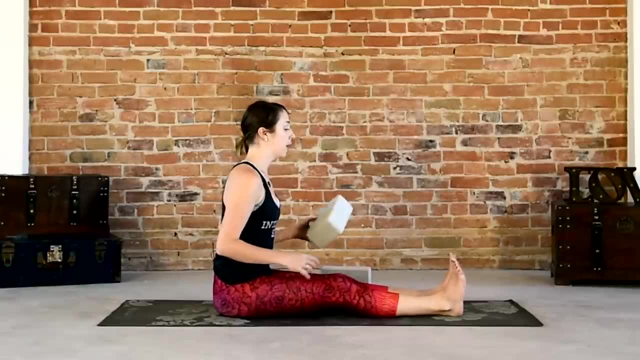 So this is the second pose- or second best pose, I find- to help relieve knots. With your blocks close by. you'll need to sit up really straight, So if you feel like you're rolling back, one of the blocks can go underneath your hips, so you have a little bit more height. 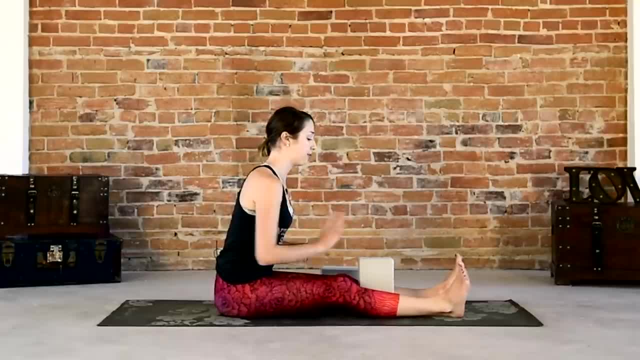 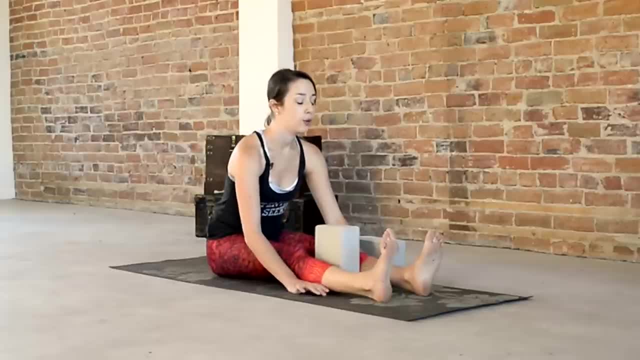 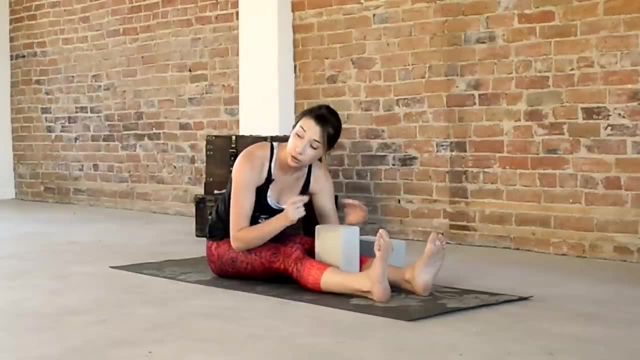 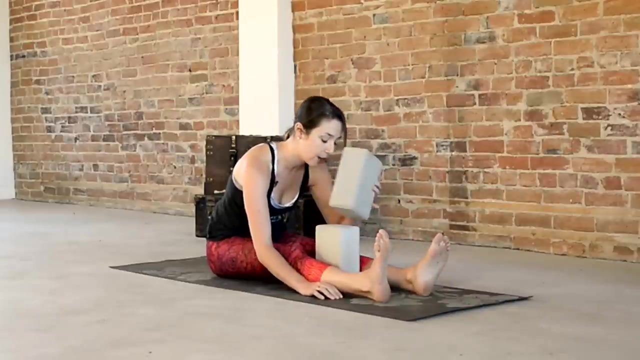 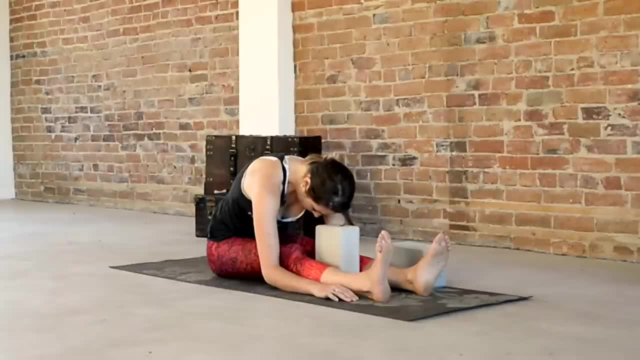 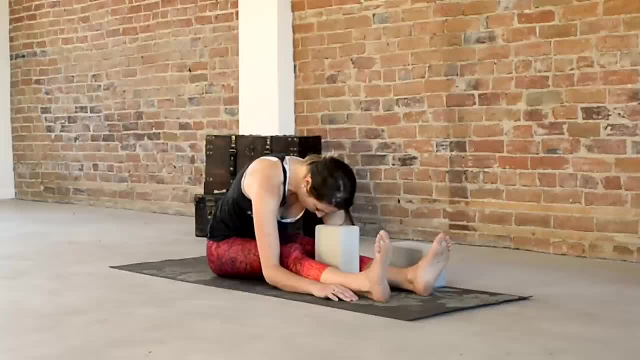 we warm up or as we go deeper into the pose, I like to put the block underneath, but you will definitely intensify the stretch along the spine if you bring your chin down. keep the shoulder blades drawing down the back, Okay, And just breathe deeply. 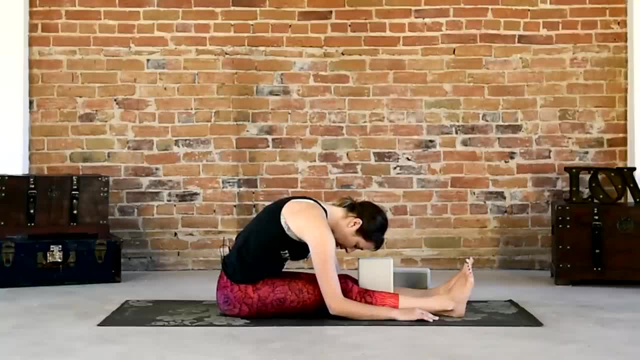 So we're not trying to push or pull here, We're letting gravity do the work, Even feel the arms, relaxing the jaw, the facial muscles. So we're not trying to push or pull here, We're letting gravity do the work. 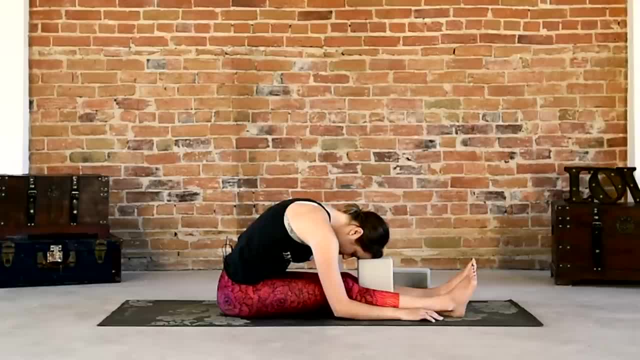 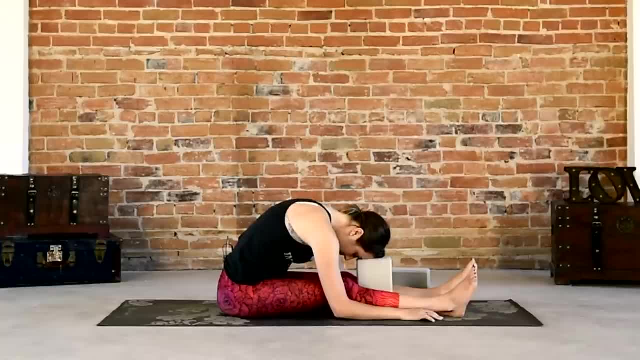 So we're not trying to push or pull here. Notice if your breath is short or shallow, Try to keep it long and smooth in and out through the nose. So we're really deeply stretching through the entire posterior chain, which is the crown of the head down the spine. 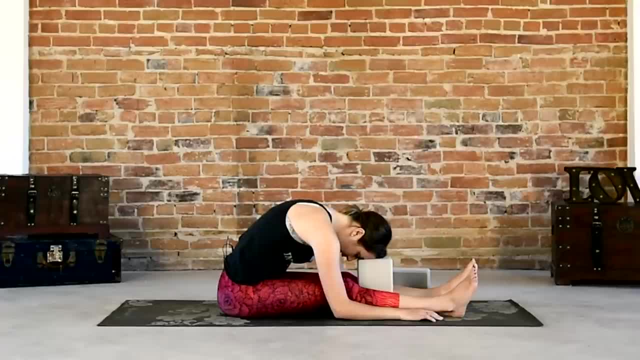 and all the way down the legs and the hamstrings and calves. So imagine your breath can travel down this channel every time you inhale. and every time you exhale, holding for about another minute or so. And as you inhale, hold for about another minute or so. 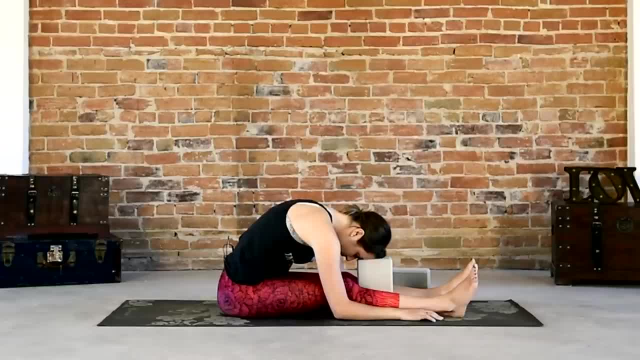 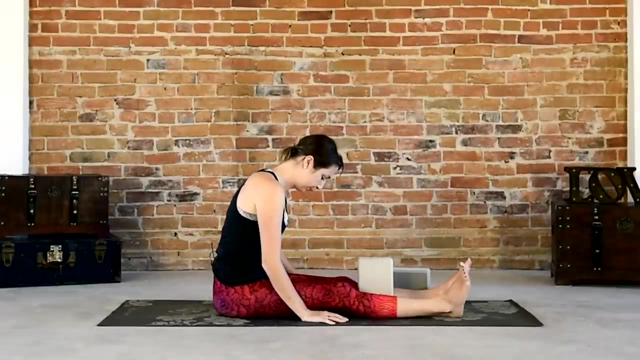 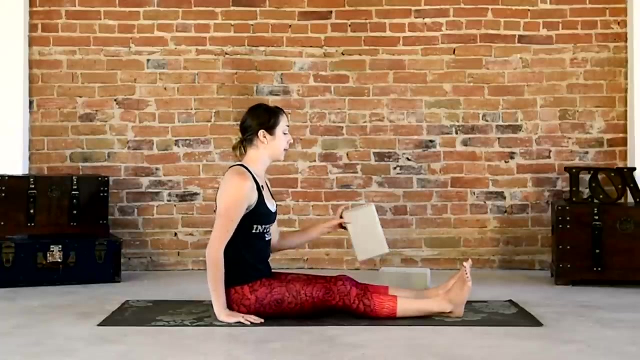 And, as you exhale, hold for about another minute or so. Try to use mostly arm strength and go inch by inch. There's no need to rush this. Keep breathing even as you unwind- Going nice and slow- And a really great way to release after a deep forward fold like this one is to take a twist. 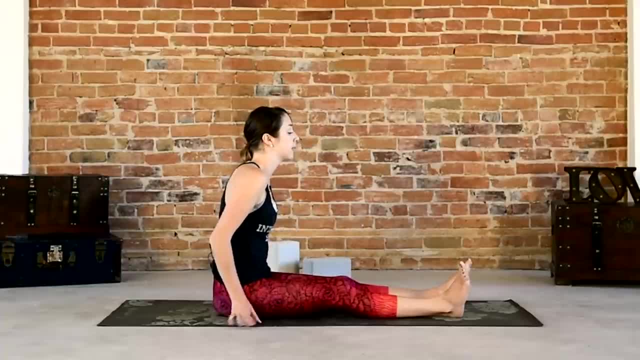 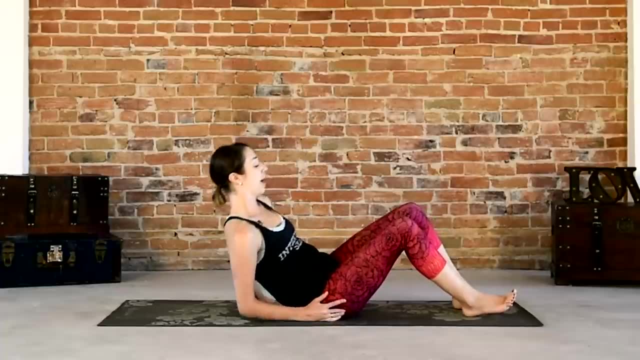 And this is great for the upper back as well. So we're going to lie down on our backs Our final pose before we come into Shavasana. We'll take a Lange's final twist, So let yourself roll all the way back down with your knees bent, feet flat to the floor. 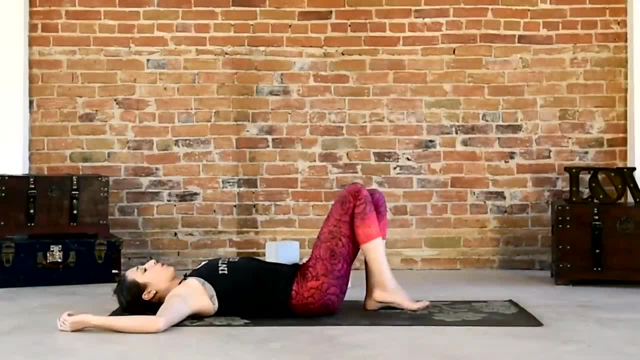 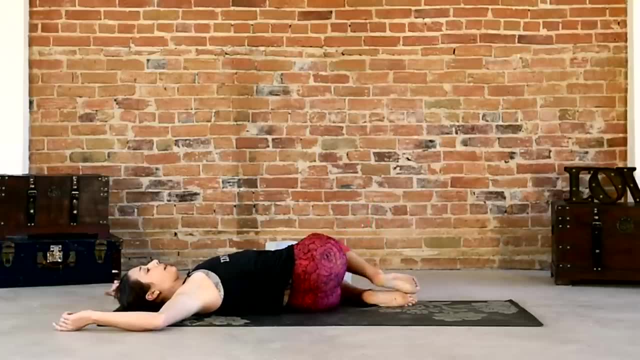 Go ahead and reach the arms out to the sides. You're going to press your feet to the ground in order to lift your hips and shift them over to the right, Both knees dropping down to the left, Either just keeping one leg over the top of the other. 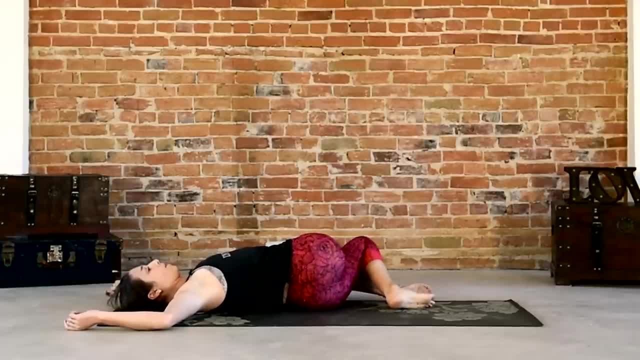 or you can always intensify this by crossing one thigh- your right thigh- over the left. So really, what's mostly important is that you're keeping both shoulder blades grounded on the floor. Gaze can be straight up or even looking towards your right shoulder. 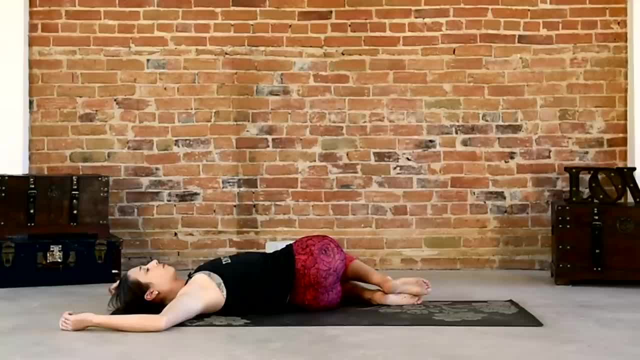 And you're going to see that your upper back línea or your left leg are being supported. So just keep a straight, straight, straight entry. This time we're going to go down to your hips, So you're going to bring your right leg up. 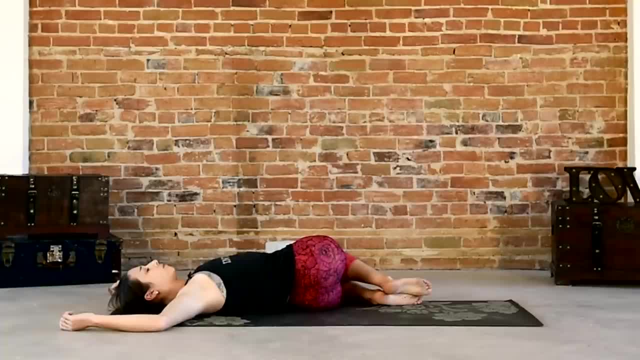 Just hold that back, And if you're not ready yet, you've got a good chance. you're going to be able to do this. So if you're not ready, you're the same. Maybe you hit your head or you're not ready yet. 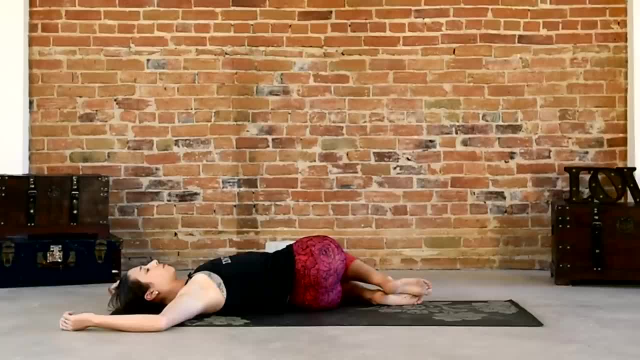 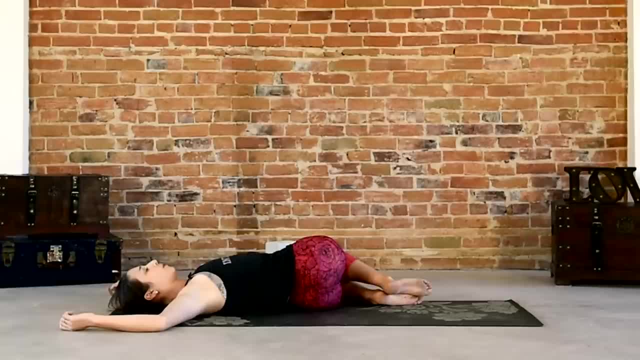 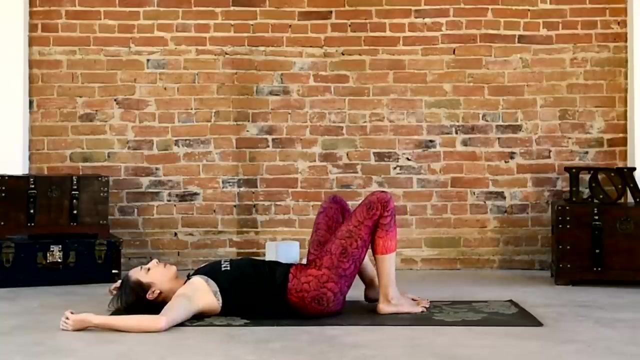 on the area of your back that's causing pain or discomfort. Thank you, Engaging the belly. Pull the knees back up, one at a time. We'll make our way to the other side, so this time the hips slide to the left. 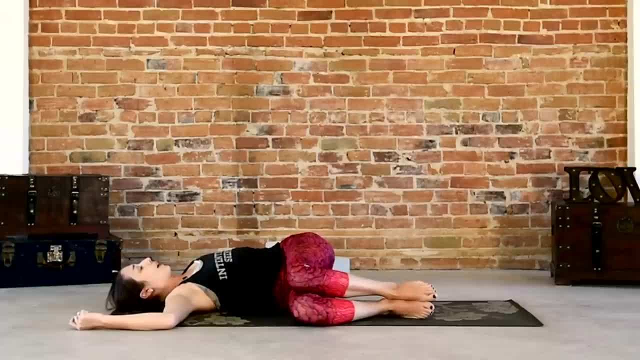 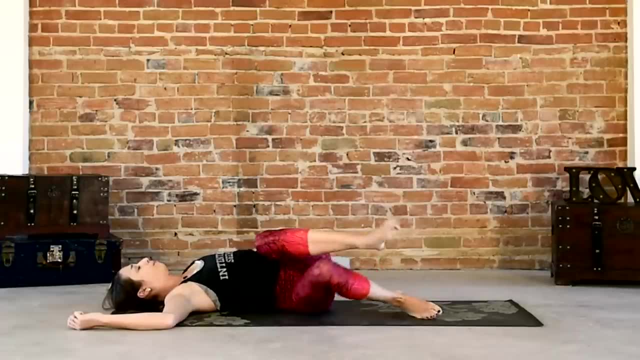 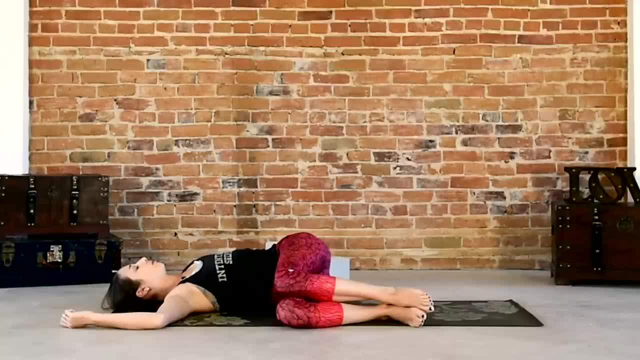 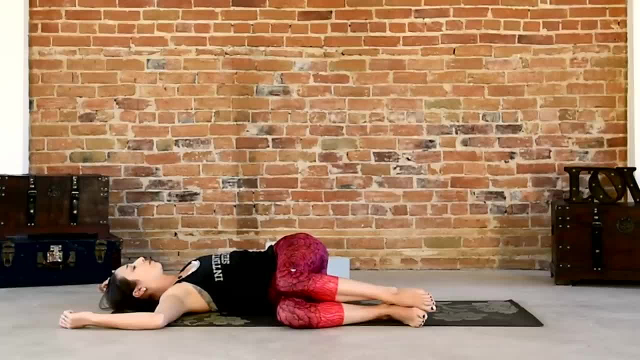